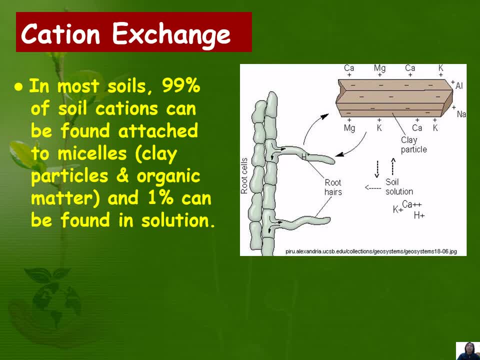 In most soils, 99% of soil cation ions can be found. This is the process of Cation Exchange. In the video you can see the figure with my finger once again. So you see here this, our picture of the soil solution that is attached to micele. 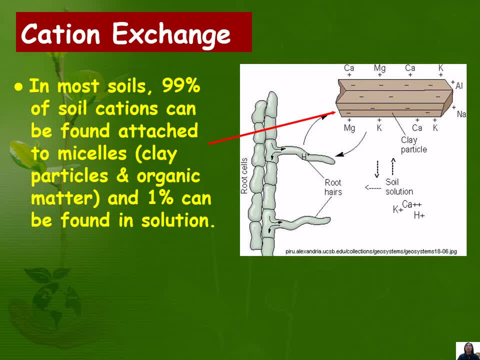 Those miceles are the clay particles and the organic matter, and 1% can be found in the soil solution. In the arrow you can see that there is an illustration of clay particles with attached or absorbed that ions such as theossium, magnesium, aluminum and sodium. 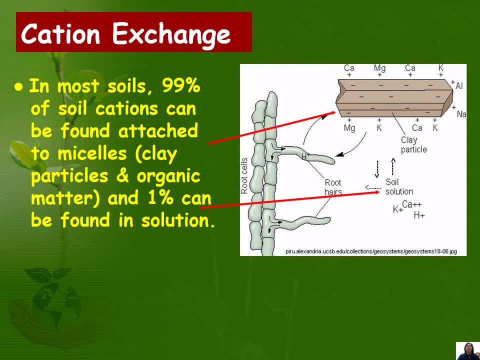 and This is the arrow for the soil solution, where you can find also the ions for potassium, calcium and hydrogen. Now, the soil solution is the water surrounding soil particles, which contain dissolved minerals and salts. So, as you can see, cation exchange is not only happening between the soil solution and the clay particle. 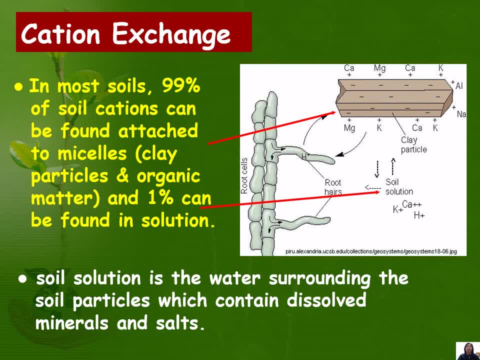 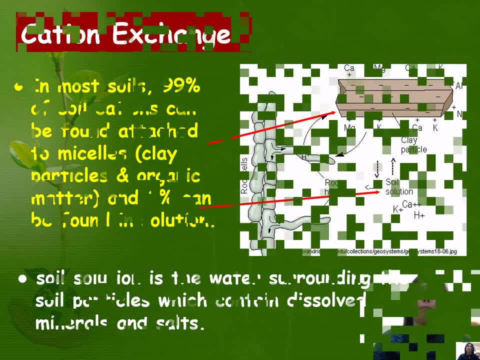 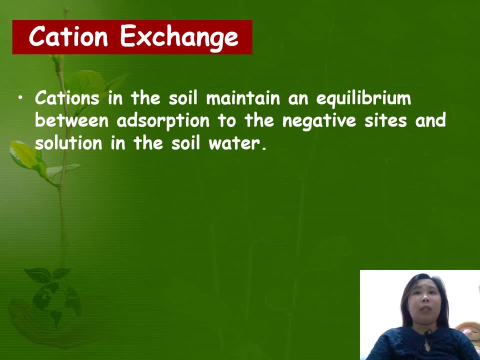 It can also be between the root hairs or the plant roots and the soil solution and or the clay particles. Cations in the soil maintain an equilibrium between adsorption to the negative sites and solution in the soil water, And this equilibrium produces exchanges When one cation detaches from a site. 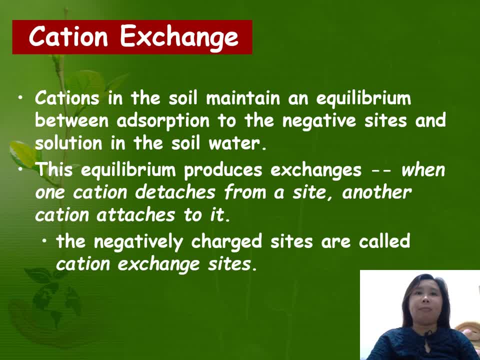 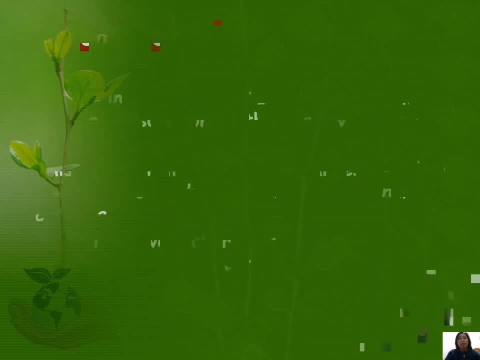 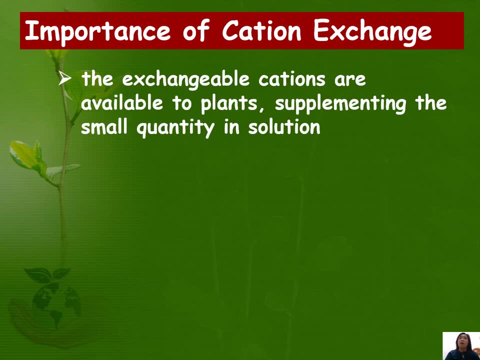 another cation attaches to it, And the negatively charged sites are called cation exchange sites. This is the importance of cation exchange. Why are we studying cation exchange Number one? it's because the exchangeable cations are being made available to plants. 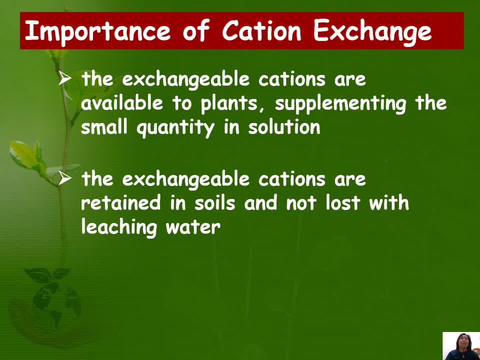 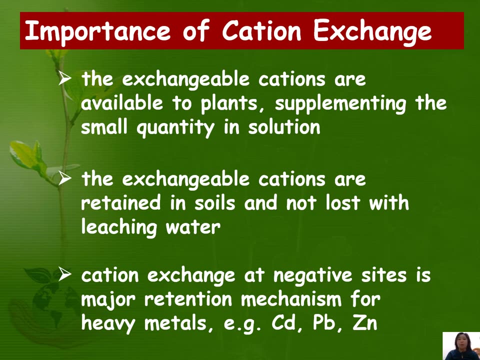 supplementing the small quantity in solution, And also those cations are retained in the soil And not lost with leaching water. Another importance is that cation exchange at negative sites is a major attention mechanism for heavy metals such as cadmium, lead and zinc. 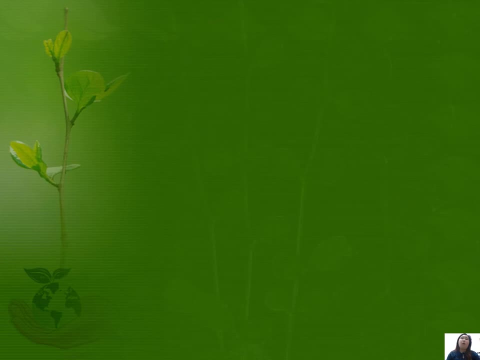 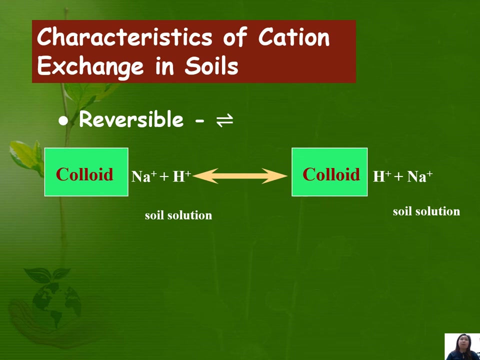 Now we are moving on with the characteristics of cation exchange in soils. Number one characteristic is that it is reversible. For example, you have a cation exchange in soil. For example, you have a cation exchange in soil, You have this sodium ion adsorbed in the soil colloid and hydrogen ion present in the soil solution. 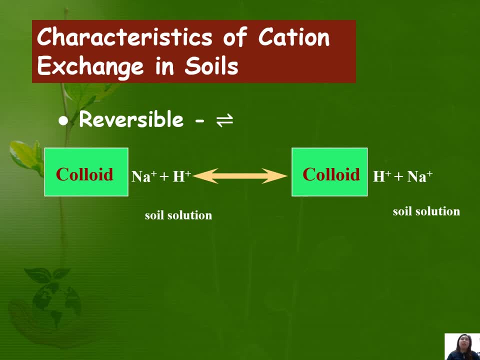 When the exchange can happen to the right. hydrogen ions could be attached or adsorbed in the colloid, And this time the sodium is in the soil solution. This process could be reversible. It could happen to the right or to the left. 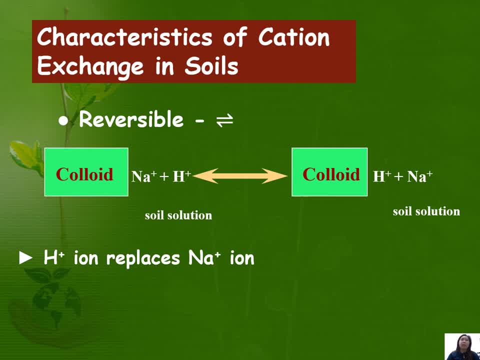 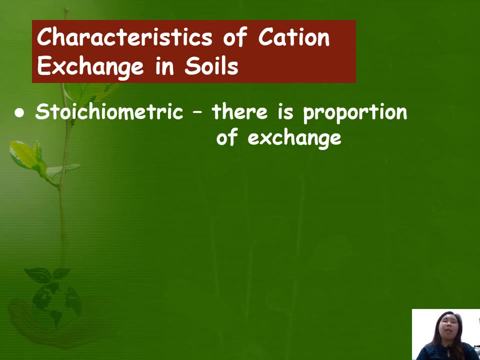 This process could be reversible. It could happen to the right or to the left. Hydrogen ion replaces the sodium ion and reaction will go to the left if the sodium is added to the system. Another characteristic is that it is stoichiometric, meaning there is proportion of exchange. 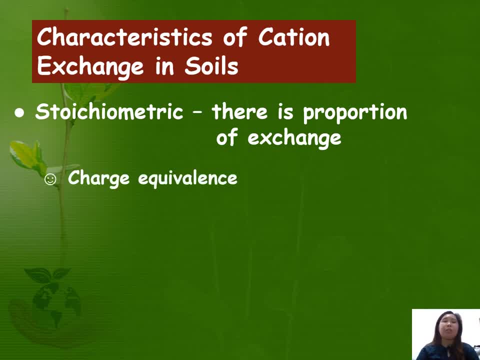 It is in consideration with the charge prevalence and the exchange is chemically equivalent. It takes the life time of the change. It takes the life time of the change. It takes place on a charge-for-charge basis. An example is that one calcium ion, calcium 2+, will replace two hydrogen ions. 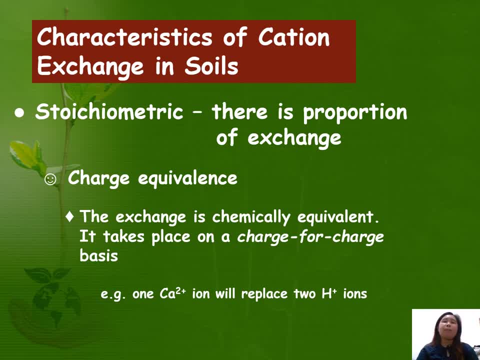 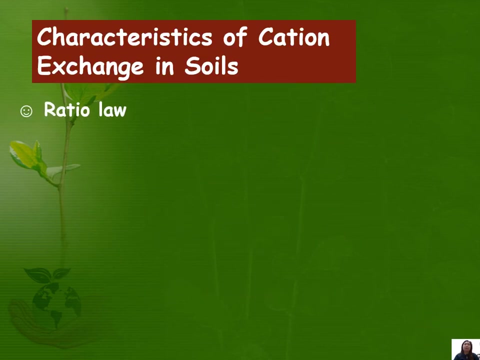 Meaning there should be a charge equivalent. It should be chemically equivalent. For example, one magnesium ion, magnesium 2+, will replace two hydrogen ions or H+. Another characteristic is the ratio law. It is following a ratio law, For example, calcium 2+ and magnesium 2+. 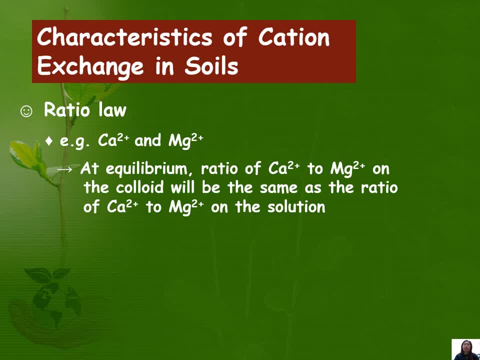 At equilibrium, ratio of calcium 2+ to magnesium 2+ on the Colloid will be the same as the ratio of calcium 2+ to magnesium 2+ on the Soil solution. For example, this ratio for calcium is to one magnesium. 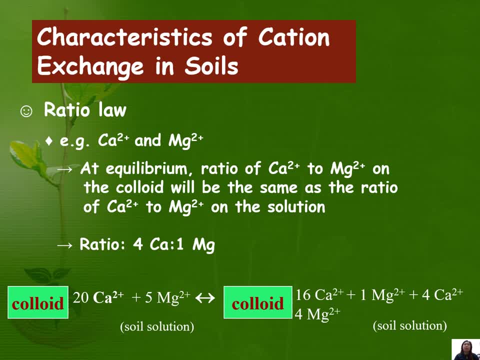 So this is an example of the chemical reaction. There is 20 calcium 2+ adsorbed in the colloid and five magnesium 2+ That is present in the soil solution. When exchange- a cation exchange- happens, it should have this same ratio against or compared to the previous one before the exchange process begins. 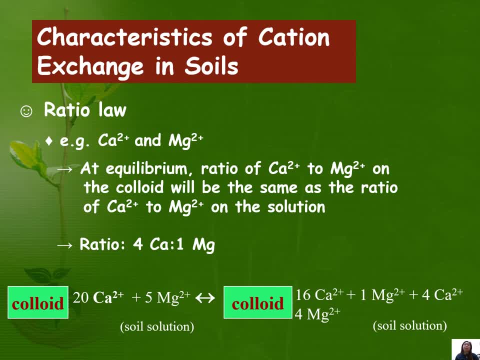 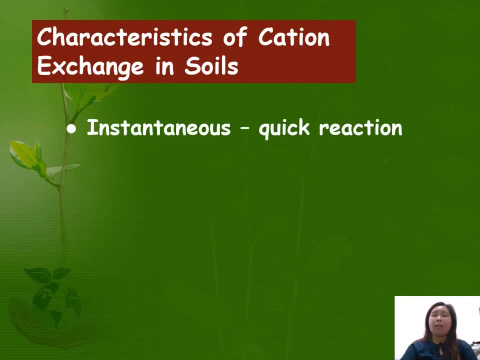 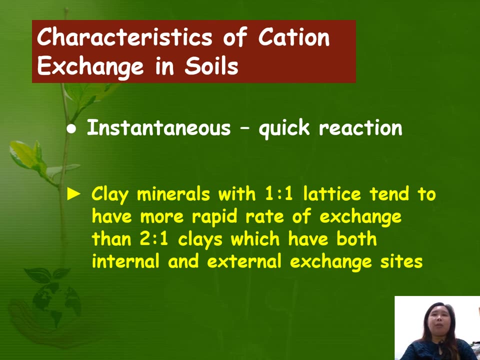 The ratio would still be 4. calcium is to 1 magnesium. Another characteristic of another solution is the count. It is a kind of a power ratio. is that the reaction is instantaneous or there is a quick reaction? clay minerals with 1 is to 1. 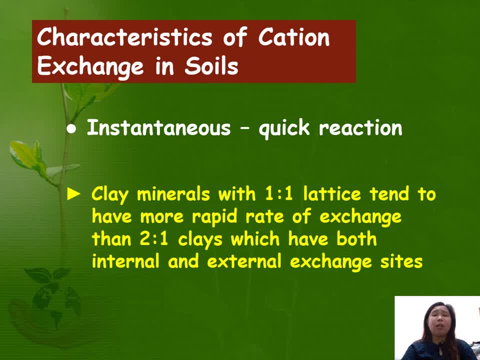 lattice, tend to have more rapid rate of exchange than 2 is to 1 clays, which have both internal and external exchange size. so, as you can, if you can remember when we study or when we discuss about 1 is to 1 clay minerals such as the kandites. the most dominant or prominent example of kandite is 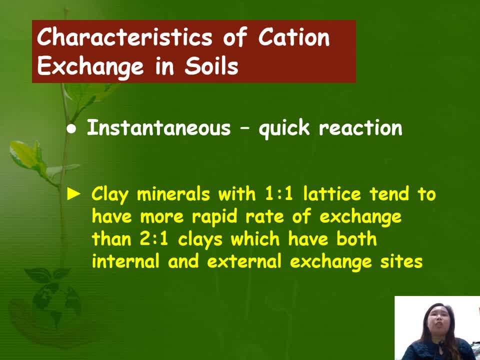 the kalenite. the exchange rate is more rapid on those 1 is to 1 clay hollows and those that are 2 is to 1, like the montmorillonite vermiculite and elyte, because these 2 is to 1 clays have both internal and external exchanges on the. internal and external exchange rate of superclay base, and so byỗi gong andzzeridze, have a reporting from the September webinar that are benched for the earth. then the conservation of internal and external and external archiy, and then the use of the monoid process. 곳 bound does not pass the right pod як window. 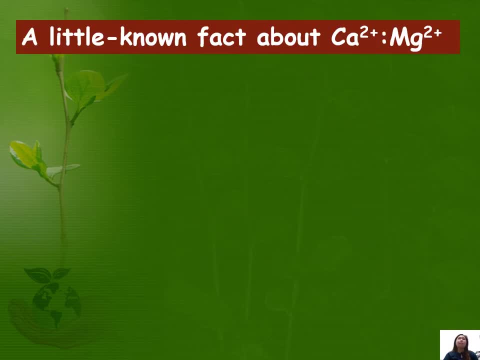 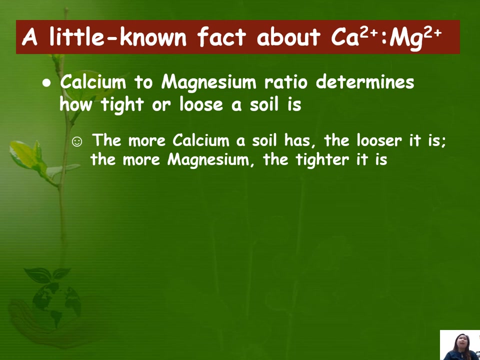 layers. There's a little known fact about calcium 2 plus and magnesium 2 plus, or the ratio of the two. Calcium to magnesium ratio determines how tight or loose a soil is. The more calcium a soil has, the looser it is and the more. 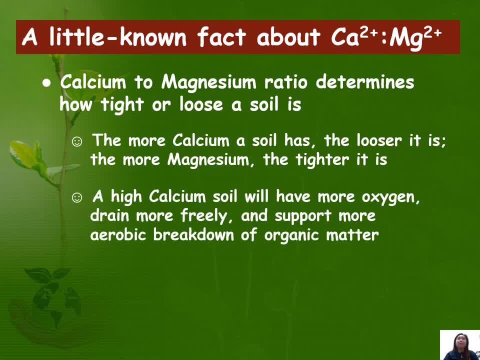 magnesium, the tighter it is. At high calcium soil will have more oxygen, drain more freely and support more aerobic breakdown of organic matter. While at high magnesium, soil will have less oxygen, tend to dry or drain slowly and organic matter will break down poorly if at all. 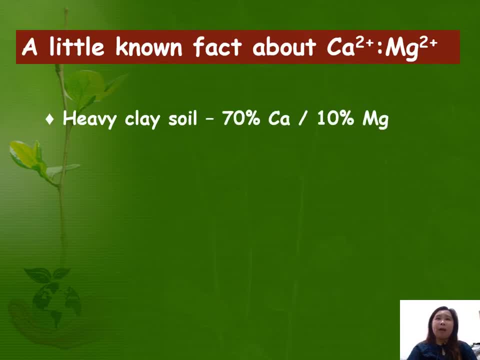 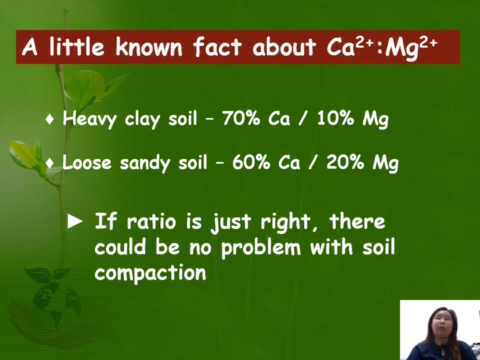 If you have heavy clay, the ratio is normally or commonly, 70 percent calcium, 10 percent magnesium. if you have a loose sandy soil, there is sixty percent calcium and twenty percent magnesium, and if the ratio is just right there could be no problem. would soil compaction Remember? the higher the 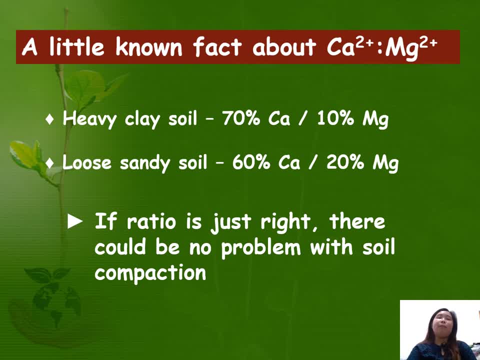 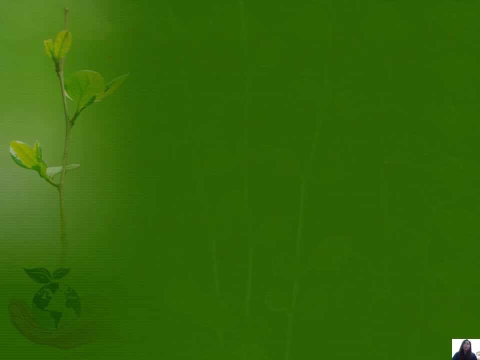 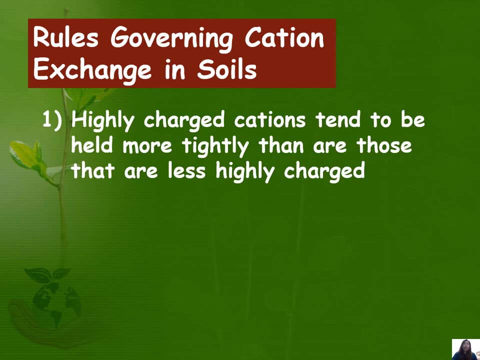 magnesium. bringt know there is no problem with soil compaction. remember, the higher the magnesium content of the soil, the soil will be more prone to compulsion. Now let's take a look on the roles governing cation exchange in soils. For rule number 1, highly charged cations tend to be held more tightly than are those that are less highly charged. 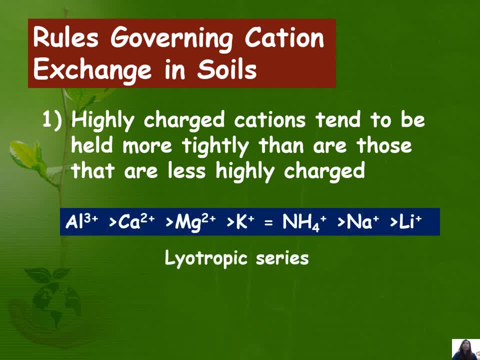 This follows this lyotropic series, wherein this lyotropic series describes the relative strength of various cations at suction. You can notice that in the lyotropic series that those cations that have high charge are more tightly held than the less highly charged. 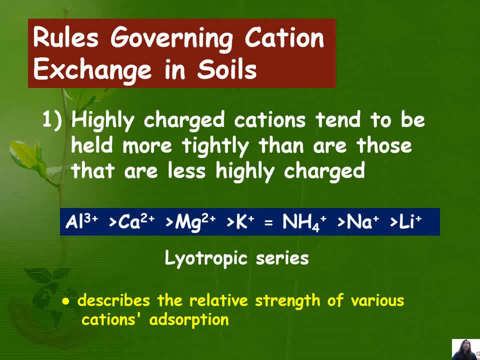 For example, Aluminum-tribe cations is more tightly held than the Calcium-2+- Magnesium-2+, and those Calcium-2+ and Magnesium-2+ are more tightly held than K+, NH-4+, Sodium-2+. 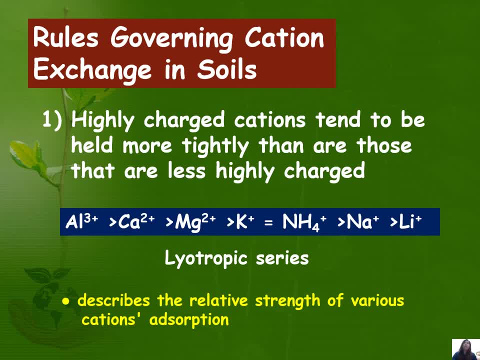 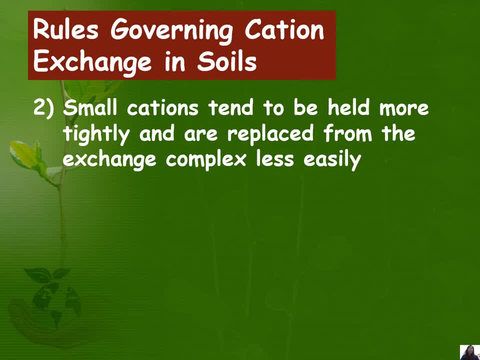 and D-3+. That's for rule number 1.. Now for rule number 2, small cations tend to be held more tightly and are less highly charged. This follows this lyotropic series showing the relative strength of the cations at suction. 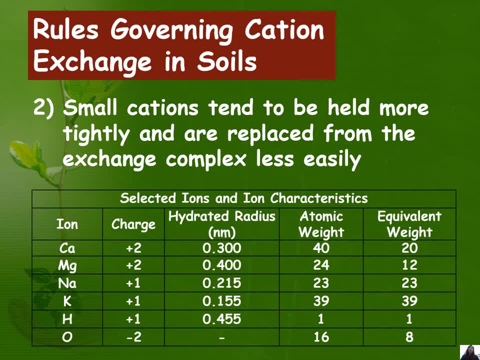 For example, Aluminum-2+, Magnesium-2+, Magnesium-2+, Sodium-2+, Sodium-2+, Sodium-2+, Magnesium-2+, Sodium-2+, Sodium-2+, Magnesium-2+, K+, K-2+. 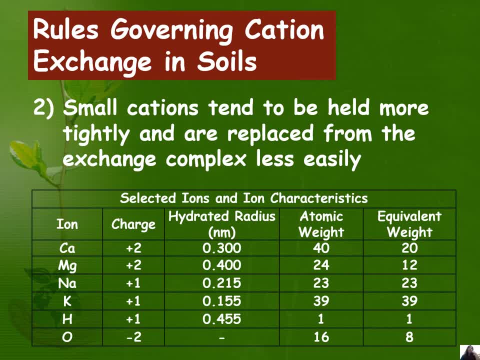 K-3+, K-3+, K-3+, K-4+, K-5,, K-6,, K-7,, K-8,, K-9,, K-11,, K-12,, K-13,, K-14,. 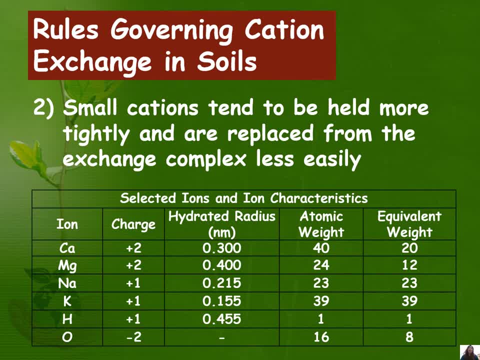 for the charge for calcium and magnesium has uh have plus two charge. sodium and potassium has have plus one charge, including hydrogen. hydrogen also has plus one, while oxygen has negative two charge. um notice, they're hydrated ratios for calcium, it has 0.300 nanometers. magnesium has 0.400 nanometers. sodium has 0.215 nanometers. potassium has 0.115. 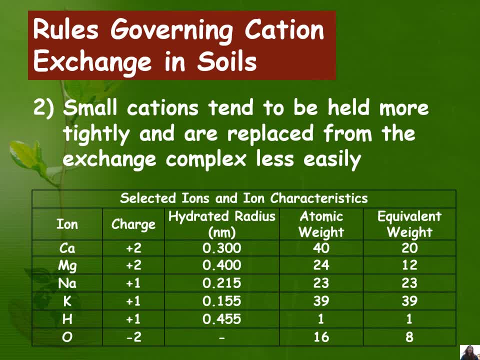 155, rather nanometers. hydrogen has 0.455 nanometers. so, based on the charge, if you can remember, the lyotropic series, calcium and emission are more tightly held than sodium, potassium and hydrogen. of course, oxygen will not be absorbed on the exchange complex because it has a negative charge. so we're just talking about the cations here, those that are. 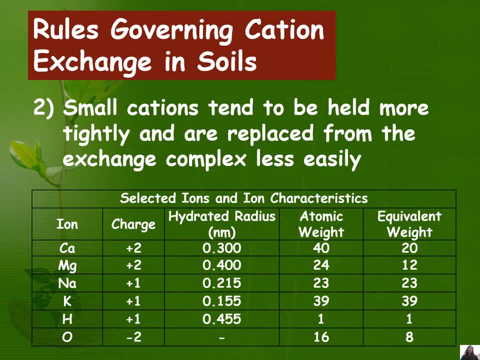 really charged. so, comparing calcium and magnesium, they both have plus two charge. but the question is which is more tightly held on the exchange complex, the calcium or the magnesium? now, based on their size, calcium is more tightly held and or are exchange or are replaced on the exchange complex. 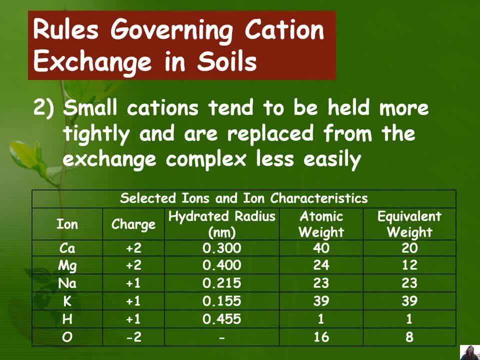 are because calcium's hydrated radius is smaller than magnesium. now another example: let's take a look on sodium, potassium and hydrogen, because these three both have possible charges. now, among these three, potassium is the smallest based on its hydrated ratios. now we can see, or we can say, that 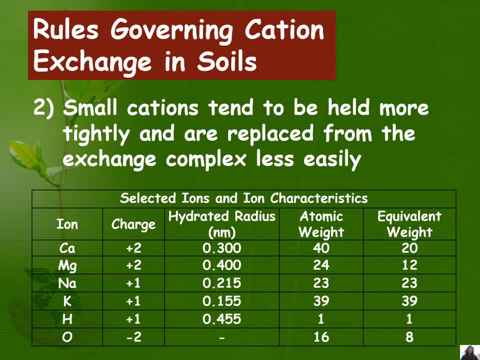 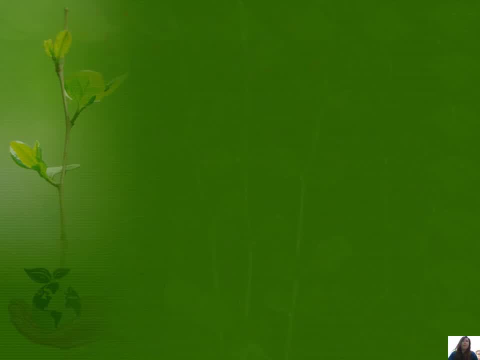 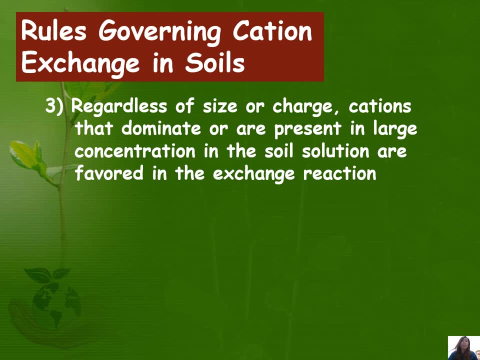 potassium is more tightly held than sodium and hydrogen because it has a small, smaller hydrated juice. now for rule number three. regardless of the size or charge, the ions that dominate or are present in large concentrations the soil solution are favored in extinction. so right now we are talking about the concentration. for rule number one, we're talking. 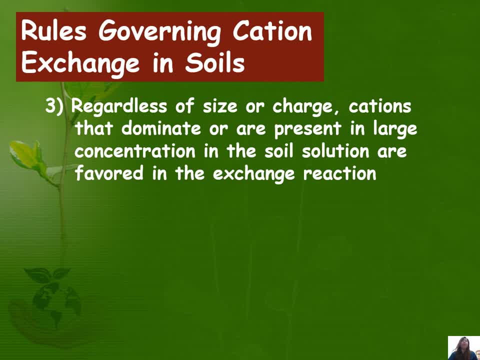 charge. rule number two: we are talking about the size, but now we are talking about concentrations, for example in very acid soils, where acid soils will have high concentrations of hydrogen and aluminum ions. so those um ions, hydrous, such as the hydrogen and aluminum ions, will be favored in the exchange uh reaction because they are present in large. 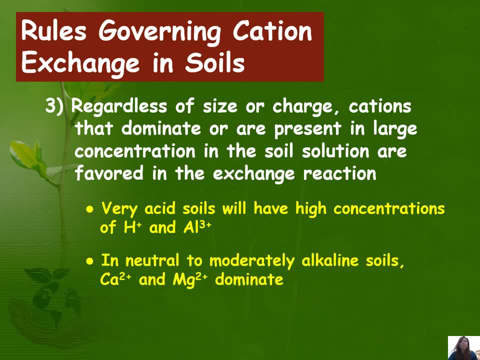 concentrations. in neutral to moderately alkaline soils, calcium and lithium ions dominate, while in poorly drained soil it may absorb sodium in very high quantities. so, based on the soil's ph and the soil's drainage or water holding capacity, you can see that you can notice that certain cations. 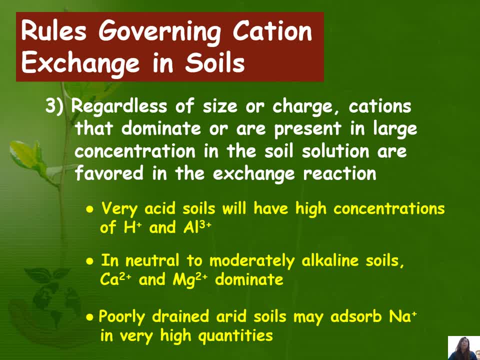 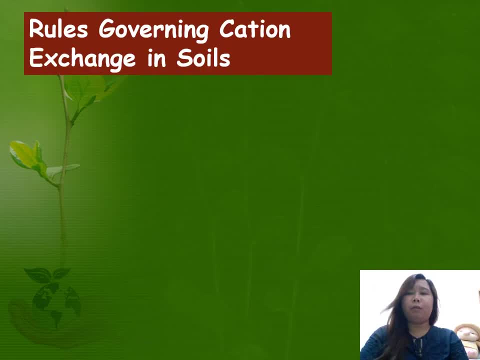 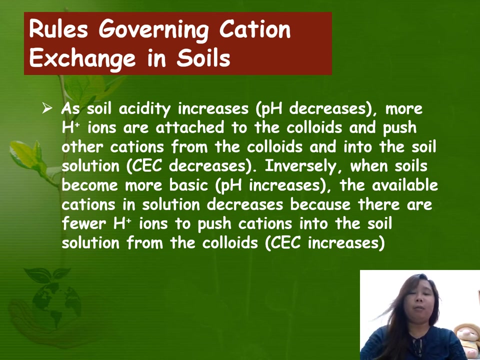 dominate, so because they are present in large concentrations, more favored in the exchange reaction. now the view can notice that lph has something to do also with the cation exchange process. the soil acidity increases, ph decreases, more hydrogen ions are attached to the colloids and push other cations from the colloids and into the soil solution. therefore the 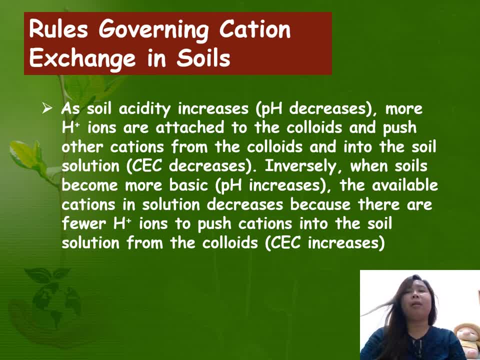 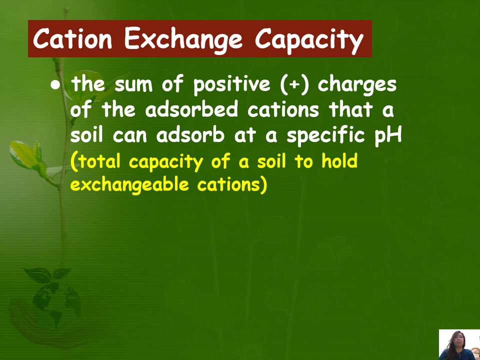 cation exchange capacity decreases inversely when soils become more basic, meaning to say ph increases, the available cations in solution decreases because there are fewer hydrogen ions to push cations into the soil solution from the colloids. therefore cec increases now now. now now, ion exchange capacity, or cec, is the sum of positive charges of the adsorb cations that a soil 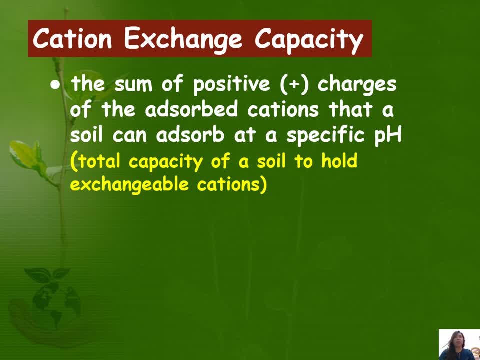 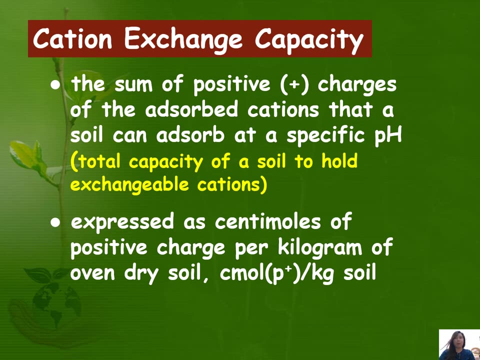 can adsorb at a specific ph, or in other words, it is the total capacity of a soil to hold exchangeable fat ions. and this cation exchange capacity can be expressed as something most of positive charge per kilogram, and that's completely true because we can tell from the level of potential chemical. 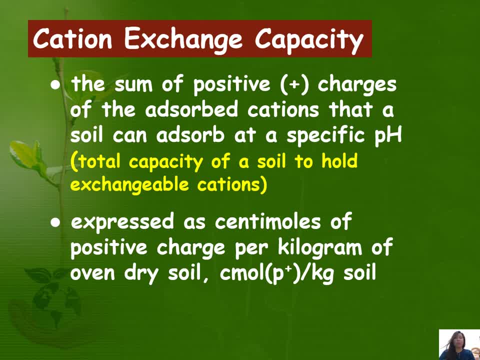 ions and bushels, and that to Non flowers andด, just as b loit, b 居 to f? kksfh soft element is another example of a level of potential chemical ions and we are going to continue on with coming out in the following steps. 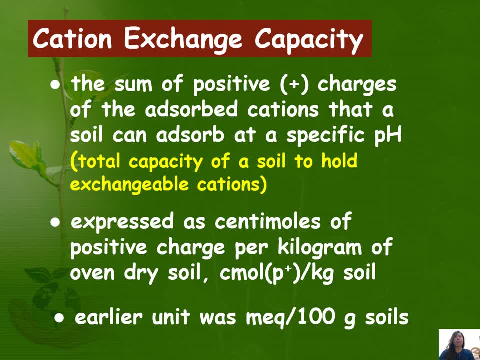 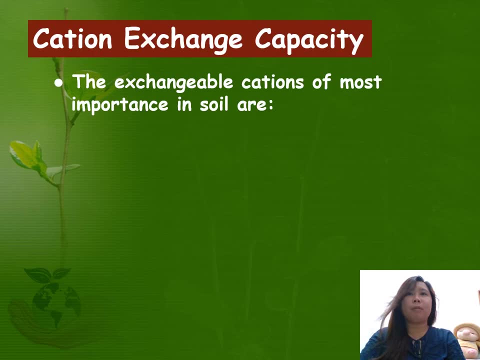 kilogram of soil um. there should be no conversion. for example, um 20 centimole per kilogram soil is just equivalent to 20 maq for 100 gram soil. how, the exchangeable cations that are most important in the soil are the following: we have 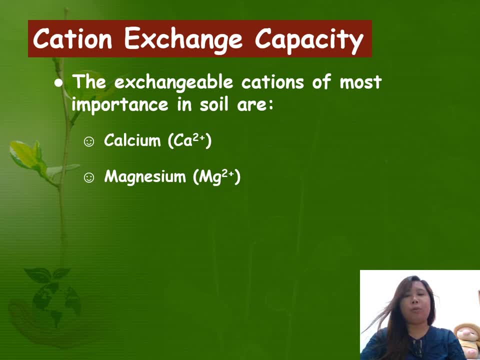 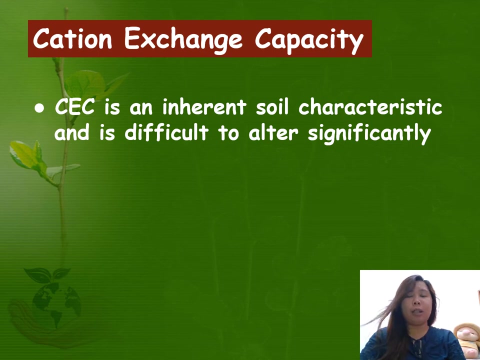 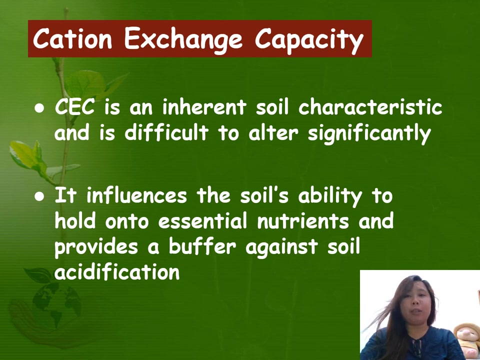 calcium 2 plus magnesium 2 plus sodium plus potassium plus and hydrogen plus. another is the aluminum 3 plus. total exchange capacity is an inherent soil characteristics and is difficult to alter significantly. it influences the soil's ability to hold on to essential nutrients and provides a buffer. 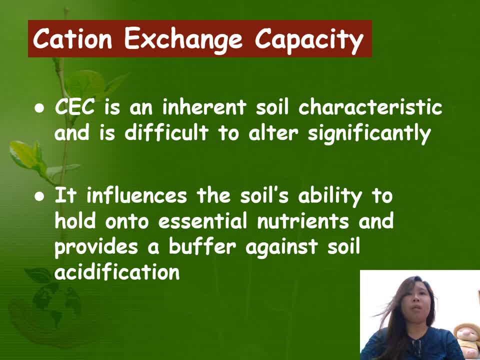 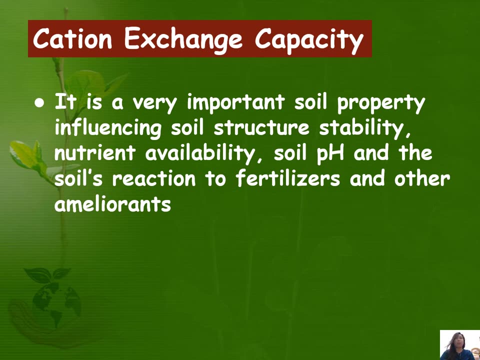 against soil acidification. so when we say essential nutrients, we are talking about essential nutrients for plant growth. it is a very important soil property influencing the soil structure, stability, nutrient availability, soil ph and the source reaction to fertilizers and other ameliorants, for example구요 a higher play fraction tend to have higher cac. 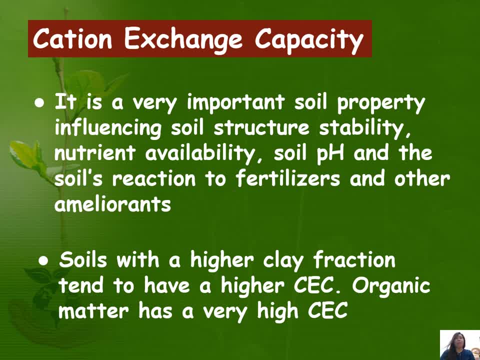 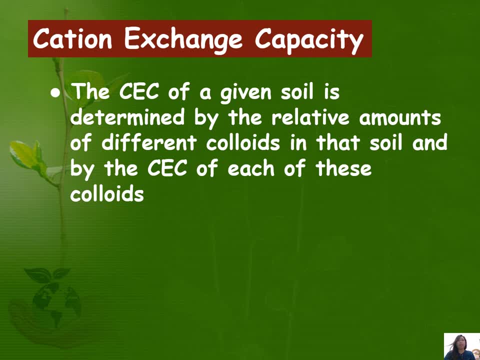 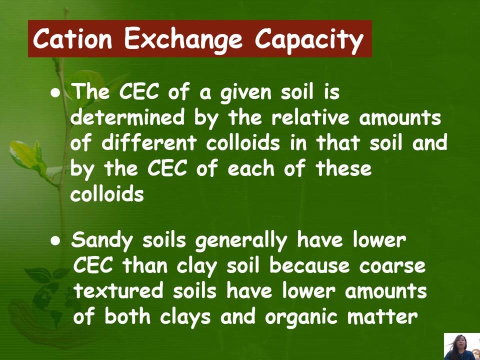 organic matter also has a very high cac. the tsc of a given soil is determined by the relative amounts of different colloids in that soil and byал the CEC of each of these colloids. For example, sandy soils generally have lower CEC than clay soil. 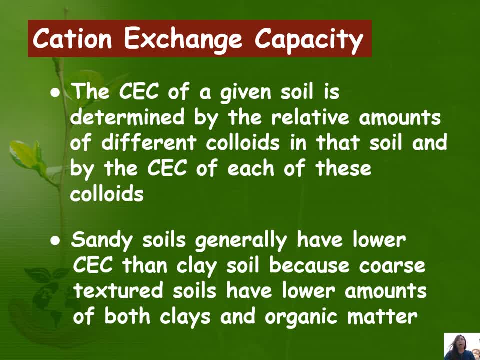 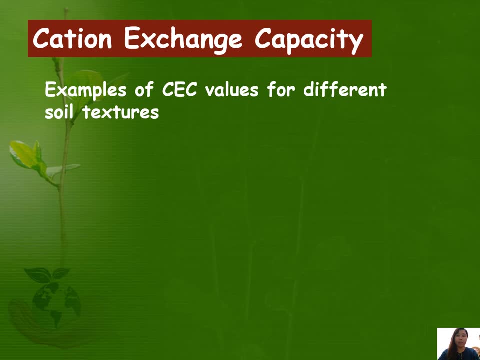 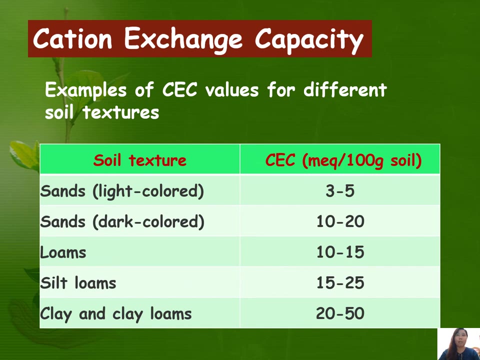 because coarse textured soils have lower content of both lace and organic matter. So in this table you can see some examples of CEC values for different soil textures. For sands that are light colored, they have 325 CEC. Sands that are dark colored have 10 to 20 CEC. 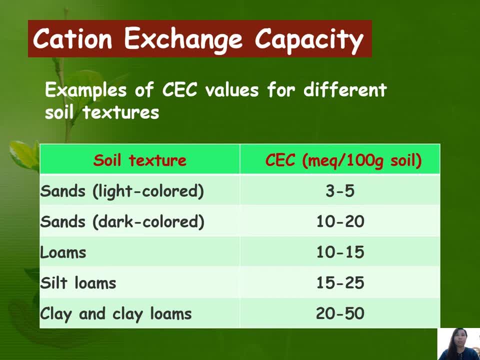 Loams have 10 to 15.. Silt loams have 15 to 25.. Clay and clay loams have 20 to 50 CEC. For sand that are light colored, they have 10 to 15.. Silt loams have 15 to 25.. Clay and clay loams have 20 to 50 CEC. 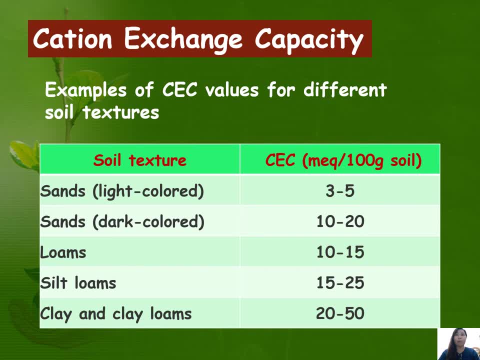 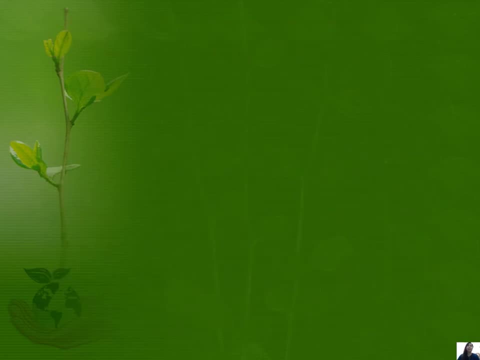 CEC, all with a unit of MEQ for 100 grams of soil. You can notice that in this examples, as the soil texture becomes finer, CEC increases. Take note of that. Now CEC is used as a measure of the soil's fertility nutrient retention. 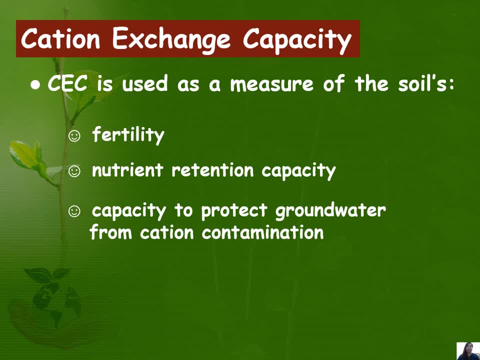 capacity- capacity to protect groundwater from cation contamination- And CEC is the measure of how much negatively charged sites are in the soil. So meaning to say the higher the CEC of the soil, the better it is for plant growth, because the higher CEC means more fertility and more nutrient retention. 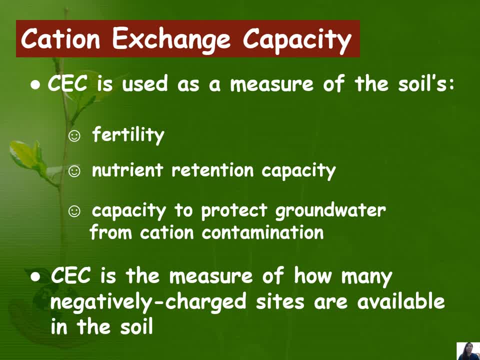 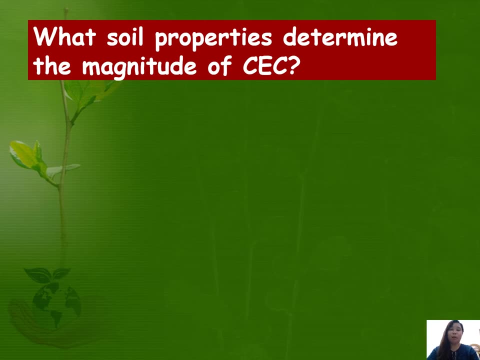 capacity in terms of protecting the environment, especially the groundwater, higher cec is desirable because it can protect the groundwater from cut iron contamination. now what soil properties determine the magnitude of cec? soil properties that determine the cec are number one. texture clay soils have higher 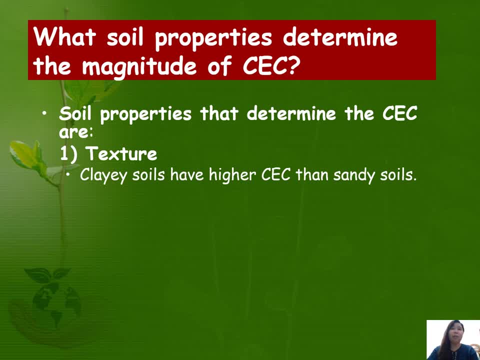 cec than sandy soils. as what i've said earlier, as the soil texture becomes finer, cec increases the amount and type of clay. mineral clay type, which is predominantly montmario unitic, has higher cec than a kalinitic clay. why? because montmario unitic has two, is the one. 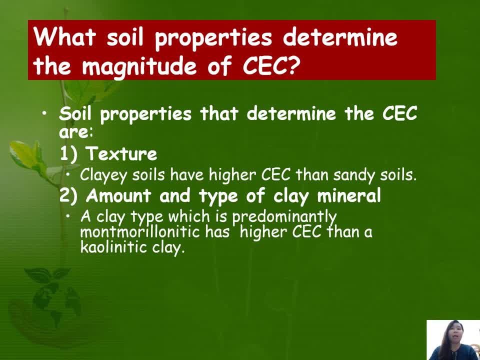 clay minerals, while kalinitic only has um. one is the one um glycolytes. so because of the interlayer space um, the more negative charge, or more negative charges are present in the two is to one clay than those that are only one is one. another is the organic matter content. 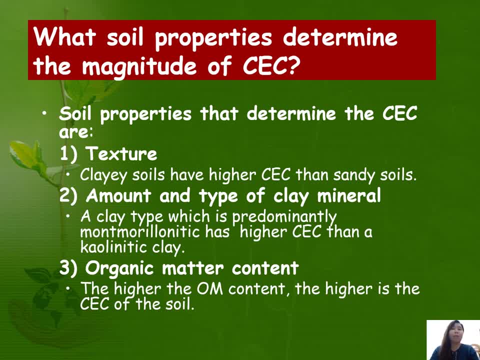 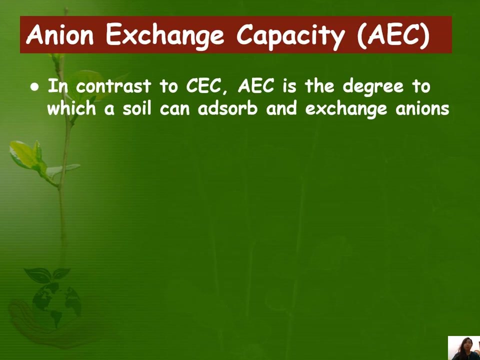 higher the organic matter content, the higher the cec of the soil that makes so. if you can remember that humus is our organic colloid and that organic colloids are, or those organic colloids are, negatively charged organic, the more organic matter content, the more you must content. therefore the higher the cec. in contrast to cec, we also have aec, which is the anion. 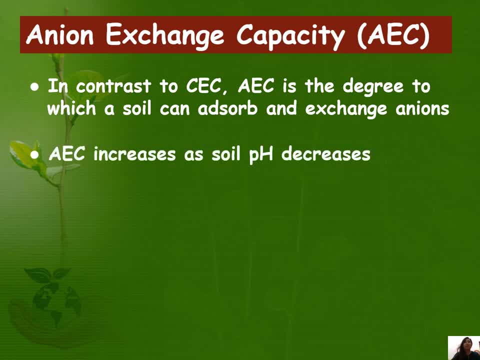 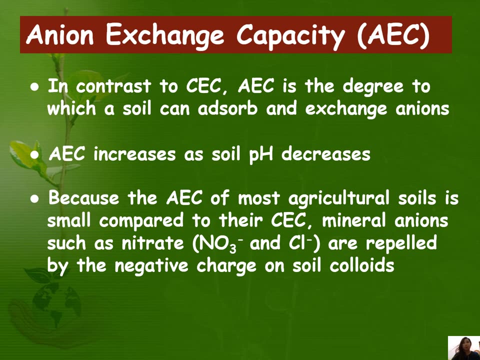 exchange capacity contrast. the cec aec is the degree to which the soil can absorb and exchange anions. aec increases as our ph decreases because the aec of most agricultural soils is small compared to their cec. mineral anions such as nitrate and chlorine are repelled by the negative charge on soil colloids. 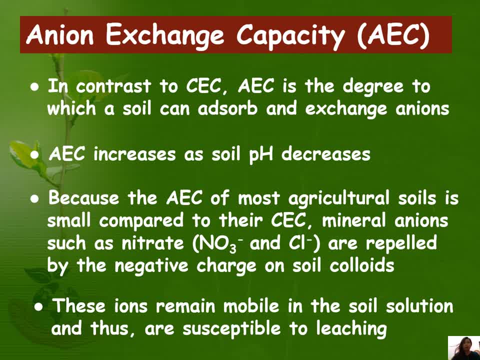 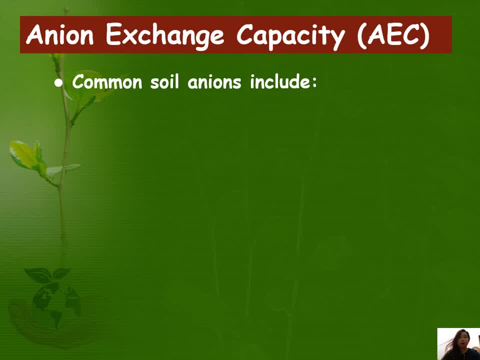 And these ions remain mobile in the soil solution and thus are susceptible to deaching. The common anions in this soil are: Chlorine, Ca- Nitrate, NO3- Sulfate, SO4-, Phosphate, PO4- And the anion lyotropic series is: 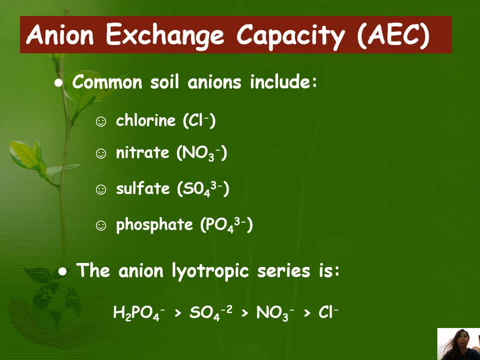 H2PO4- is greater than SO4-2, greater than NO3- greater than Cl- That is, Phosphate greater than Sulfate, greater than Nitrate, greater than Chlorine. Right now we are finished on the CEC and AEC. 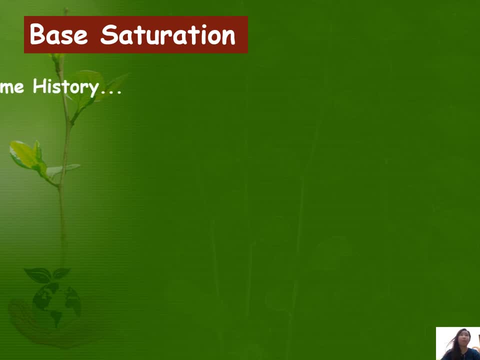 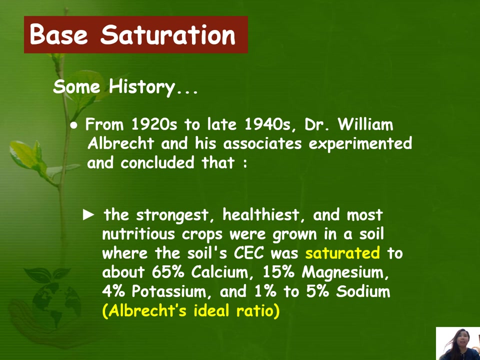 Let us now move to base saturation. To show some history: from 1920s to 1940s Dr William Albrecht and his associates experimented and concluded that the strongest, the healthiest and most nutritious crops are grown in a soil where the soil, CEC, was saturated to about 65% Calcium, 15% Magnesium, 4% Potassium and 1-5% Sodium. 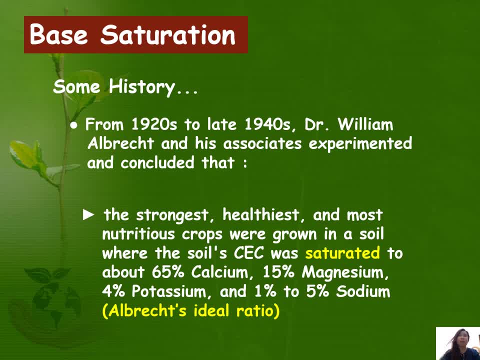 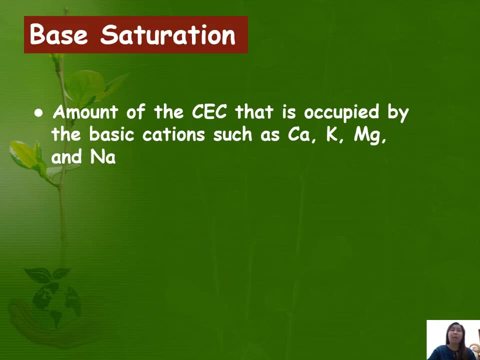 So that's the Albrecht's idea. The ratio of Calcium, Magnesium, Potassium and Sodium, which is 65,, 15,, 4, 1-5 respectively. Biosaturation refers to the amount of the CEC that is occupied by the basic cations such as Calcium, Potassium, Magnesium and Sodium. 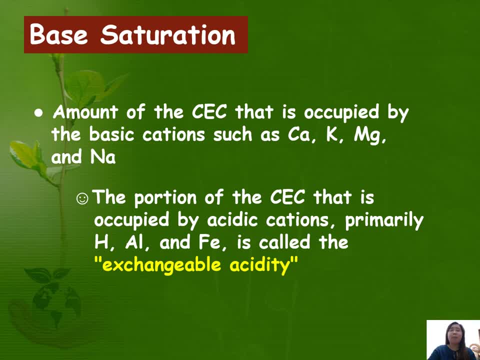 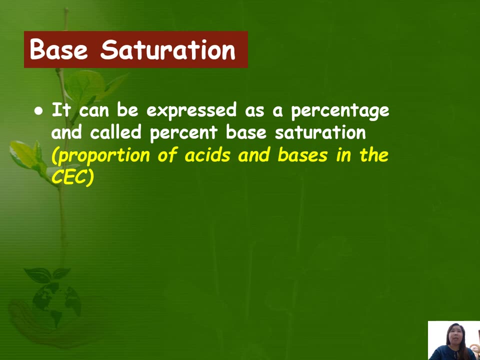 The portion of the CEC that is occupied by acidic cations, Primarily Hydrogen, Aluminium and Iron, is called the exchangeable acidity. It can be expressed as a percentage and called percent base saturation. In other words, it is the portion of acids and bases in the CEC. 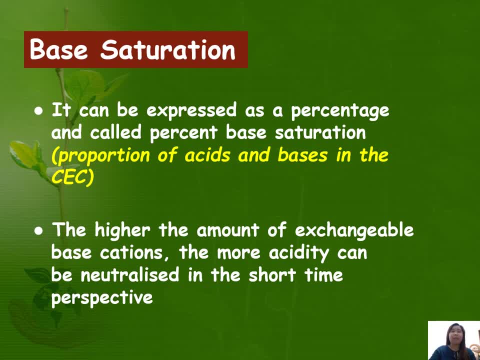 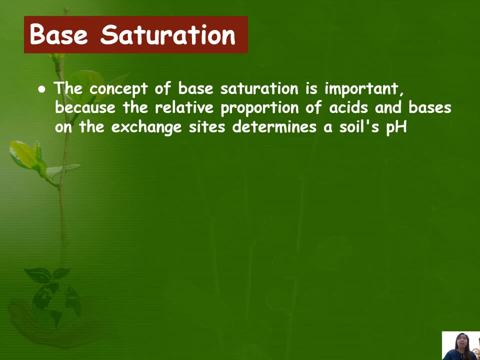 The higher the amount of exchangeable big scat ions, the more acidity can be neutralized in short-time perspective. The concept of base saturation is important because the relative proportion of acids and bases on the exchange sites determines a soil's pH. As the number of calcium and magnesium ions decreases and the number of hydrogen and aluminum ions increases, the pH drops or the soil becomes acidic. 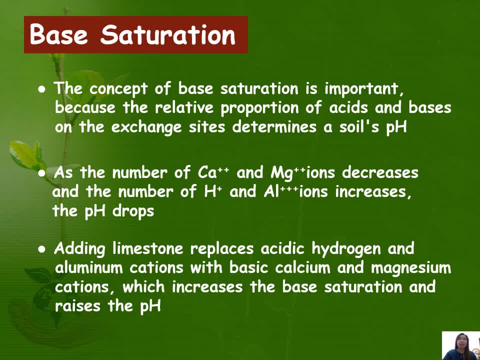 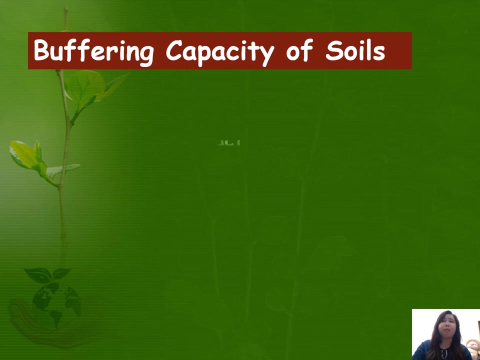 And adding limestone replaces acidic hydrogen and aluminum cations with basic calcium and magnesium cations, which increases the base saturation And therefore raises the pH. Now, in relation to base saturation, let's take a look on the buffering capacity of soils. Buffering capacity is the soil's ability to maintain a constant pH level during action on it by an acidifier or a coalescent agent. 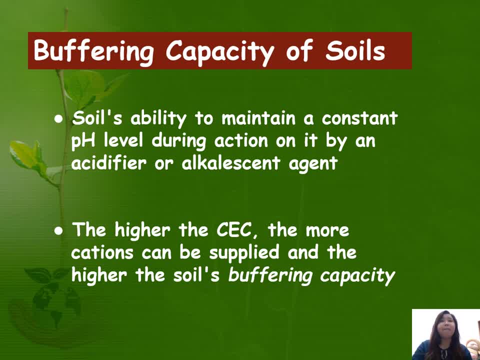 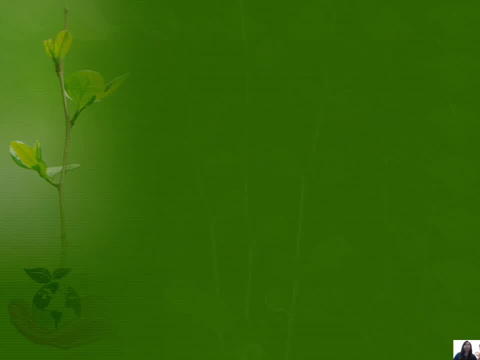 Meaning: the higher the cation exchange capacity, the more cations can be supplied and the higher the soil's buffering capacity. Now let's take a look on how to measure and estimate the cation exchange capacity. CEC can be estimated from soil texture and color. 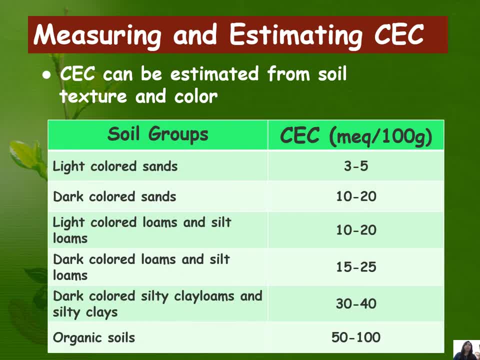 For example, in this table we have different soil groups having different soil texture and color. Light-colored sands have 3 to 5 CEC. Dark-colored sands have 10 to 20 CEC. Light-colored loams and silt loams contain 10 to 20 CEC also. 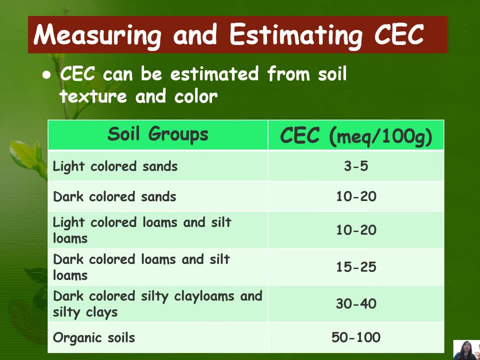 Dark-colored loams and silt loams contain 15 to 25 CEC. Dark-colored silty clay loams and silty clays have 30 to 50 CEC, While organic soils have more than 50 CEC. So notice that. 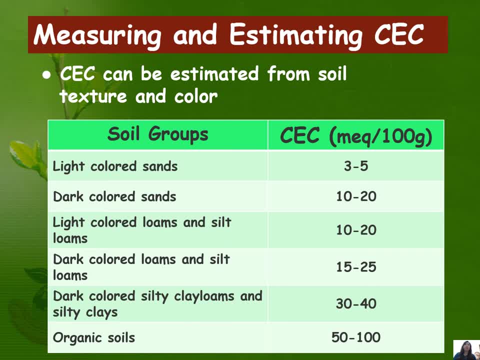 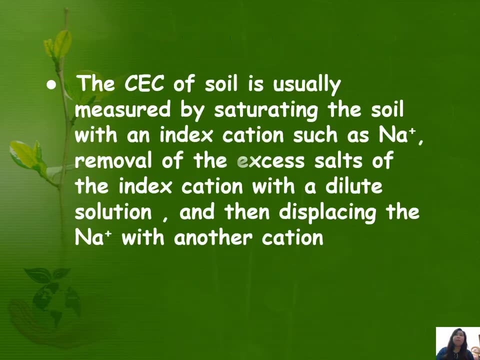 as soil color becomes darker, the higher the CEC. As the soil texture becomes finer, the higher the CEC. The higher the organic matter content, the higher the CEC. The CEC of the soil also is usually measured by saturating the soil with an index iobion. 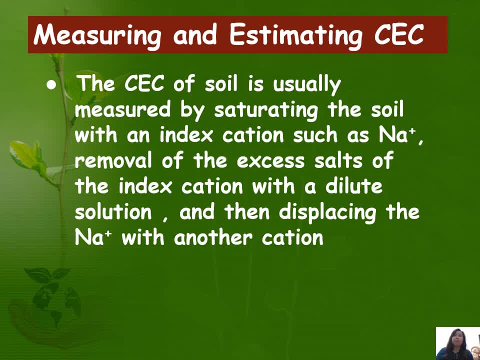 The removal of the excess salts of theisonation indexed cation with a dilute solution and then displacing the sodium ion with another cation. so this method is usually done in analytical service laboratory and the amount of sodium displaced is then measured and the CEC is calculated. now this is a sample problem, and 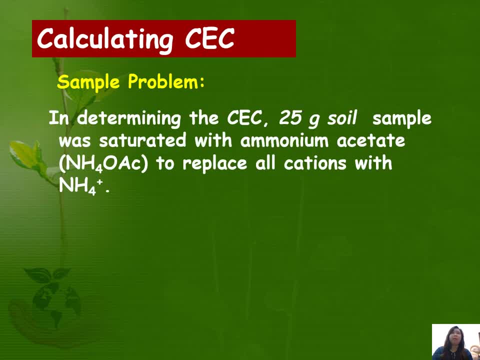 the calculation of CEC. so, for example, in determining determining the CEC, 25 grams soil sample was saturated with ammonium acetate to replace all cations with ammonium. after distillation of the ammonia, it was found that 0.07 grams of ammonium was absorbed by the soil. 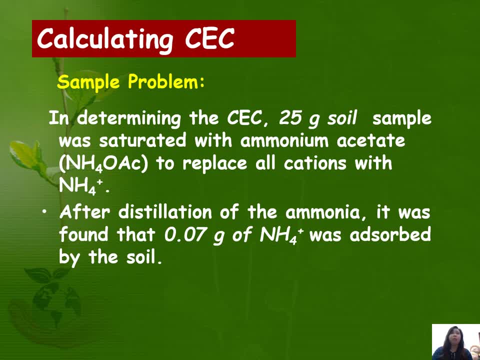 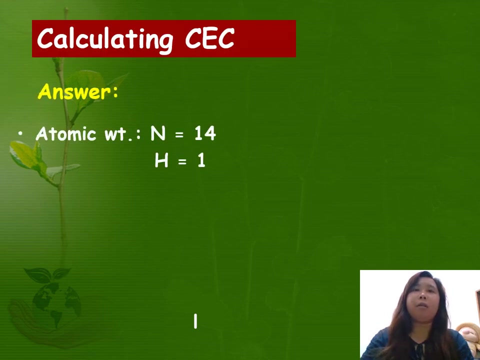 this time we use NH4 plus or ammonium to replace or displace all the cations adsorbed on the soil. now how to calculate CEC from this data? calculate the CEC from the data you have to know: the atomic weights of the nitrogen and hydrogen. 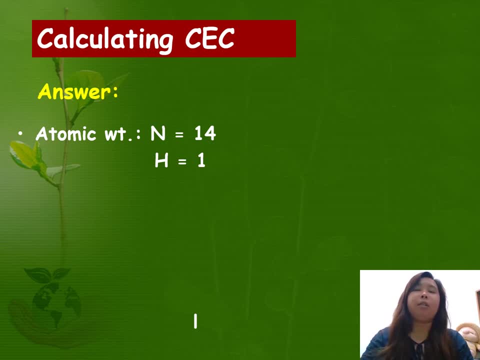 why? because that is uh, those are the cations that are present on the ammonium, the cation that is used for displacement. for nitrogen, you have 14, and for hydrogen, you have one. now let's calculate the grams per mole of ammonium, and calculate it by just summing up the atomic neat uh. 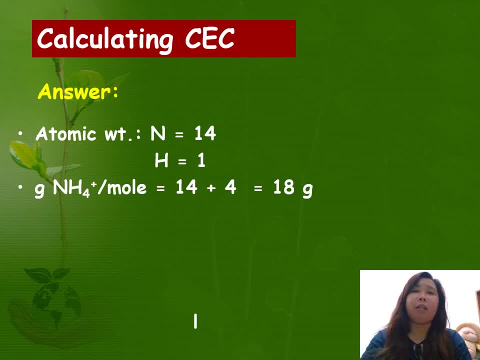 weight of the two. so 14 plus 4, you have 18 grams. now in calculating CEC, remember that the unit used is usually centimole per kilogram. so, and right now we have gram per mole, so we'll just have to convert it to grams per centimole. so just divide 18 grams by 100, you'll have 0.18 grams per centimole. 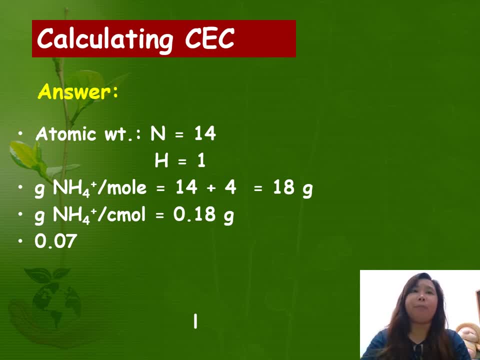 calculate the CEC to have a unit of centimole per kilogram. so, based on the data, you have 0.07 grams uh adsorbed ammonium for 25 grams of soil. let's multiply it with 0.18 grams per centimole of. 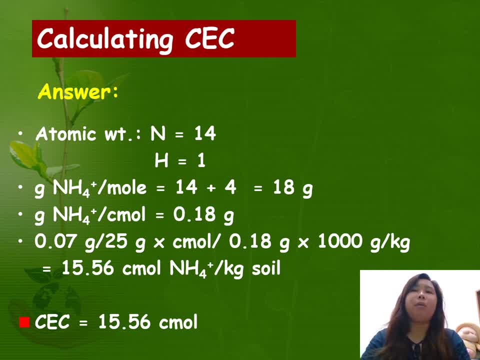 ammonium, but and also um, divided I divide it by 1000 grams to get the kilogram unit, the answer would be 15.56 centimoles of ammonium per kilogram of soil. now, since you uh, we calculated the uh amount of the CEC of ammonium. 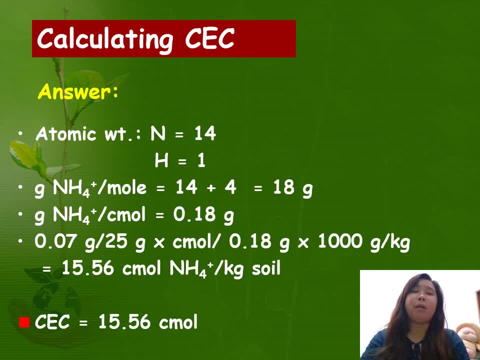 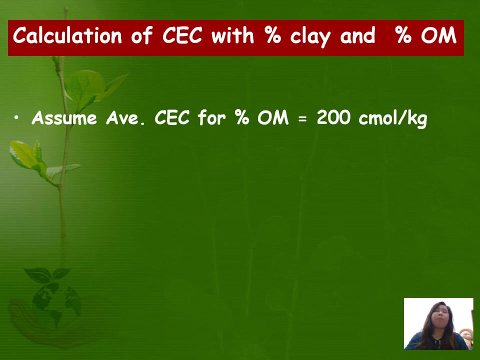 which displaces all the tonic ions present in the soil sample and that value already the answer for the total CEC of the soil. So the CEC of the soil is now 15.56 centimose ammonium per kilogram of soil. Another problem really in relation to 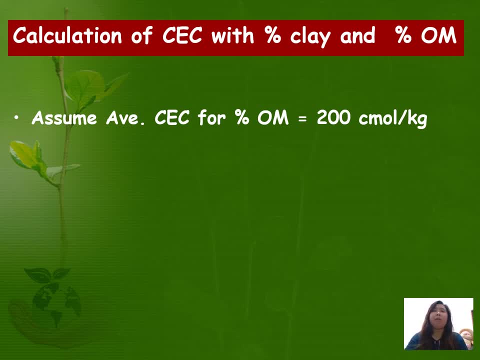 CEC or an added method in calculating CEC is when you have the data on the percent clay and percent OM organic matter content of your soil. So in calculating the CEC when you happen to have the data on the percent clay and percent organic matter of the soil, you can just assume that the average CEC for 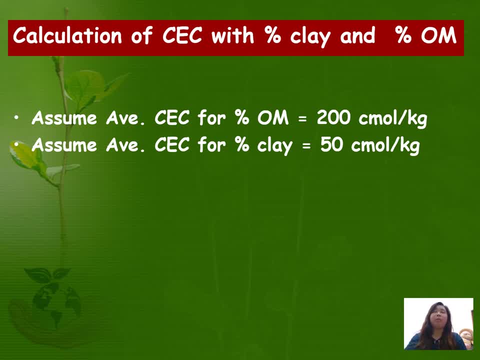 organic matter is 200 centimose per kilogram, while for the average CEC of percent clay that is 50 centimose per kilogram. Now remember that when you say clay, it could be montmorillonite, smectite, kilinite, elite chloride or organic colloids. 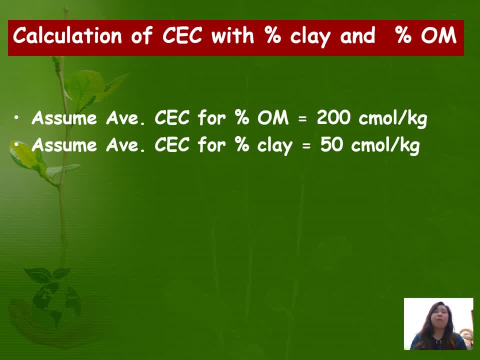 or rather inorganic colloids. so remember those five. so, on the data, we don't know right now what kind of clay colloids we are talking about, but we can just safely assume that the average CEC per percent clay, regardless of what is the dominant clay for the soil sample, is present. 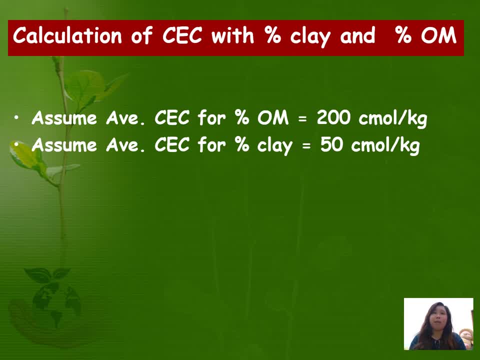 you can just use the average CEC as 50-20 most per kilogram. so the formula for CEC. but in using the percent organic matter and percentage, this CEC is equal to percent organic matter times 200. that is the average CEC for organic matter content. 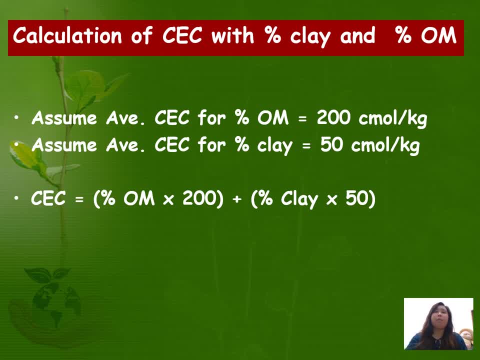 or for organic matter, rather plus percent clay times 50, that is the average CEC for percent clay. so from soil data, for example, you have the data from the laboratory on on OM and clay content. so in this example we have two percent organic matter and 10 percent clay. so to calculate CEC, 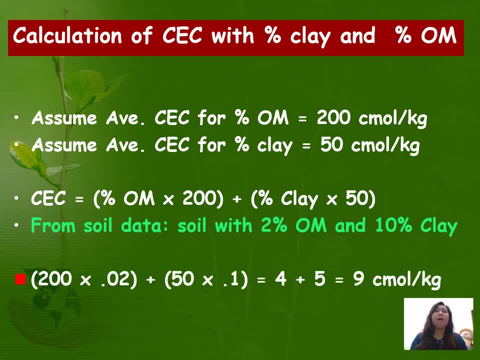 you just have to plug in the data. we'll have 220. most organic matter times 0.02. that is, from the 2% organic matter content. organic matter in the soil data: 50 times 0.1. that is 0.1 is the percent clay, 10% clay. that is why it is 0.1. 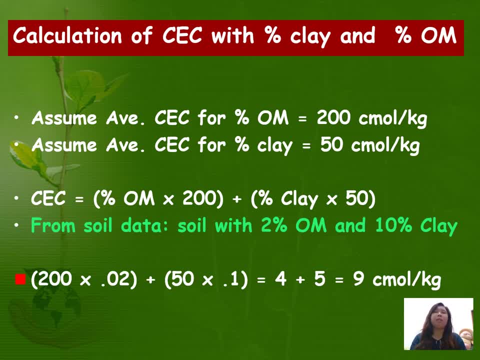 so, performing the calculation, that is 4 plus 5. the answer now for CEC is 9 centimoles per kilogram. now let's take a look on more sample problems. CEC is 9 centimoles per kilogram. now let's take a look on more sample problems. CEC is 9 centimoles per kilogram. now let's take a look on more sample problems. 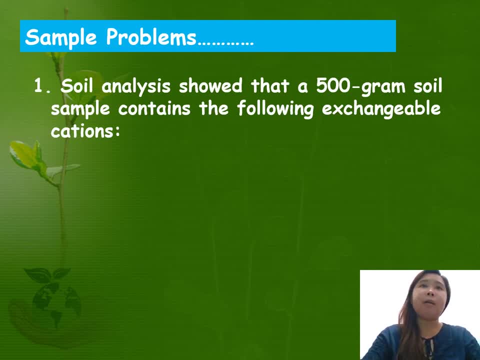 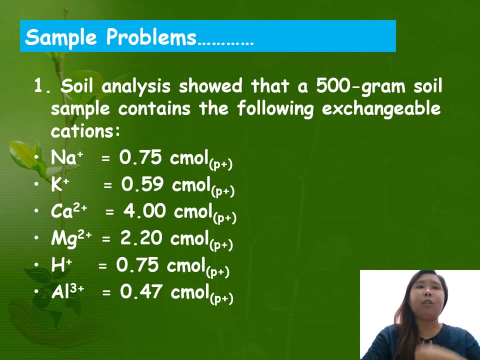 so problems? for the first problem, soil analysis showed that by 500 grams soil sample contains the following exchangeable cut ions: we have: 1.75 cmol for sodium ions, 0.59 centimole for potassium ions, 4 centimole for calcium ion. we have 1.. ponieważ ions centimole point friendians, centimole for munition, ions 1.70 point centimole for June, ions 1.97 centimole for potassium ions four centimole for iron, 2 more centimole for calcio and 2 point point 20 centimole 就опERY Cabells, Coroyerions, Calcium Ch, Thanos, Bases, Darien's, Potassium iodine Oxygen. 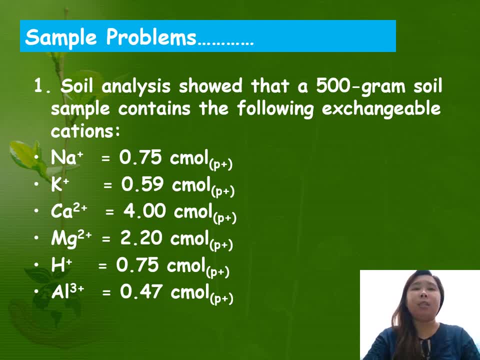 sent old mission ions. one seventy-two centimole for malicious ions is 4.2 centimole for balloons or Southern ions- a small fraction of the Colombians in Soga mo manufacturingzan 0.75 centimoles for hydrogen ions and 0.47 centimoles for aluminum chips. so the calculate. 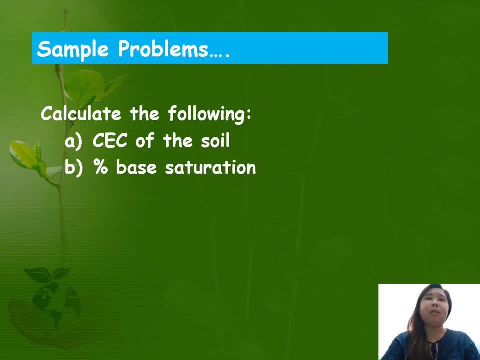 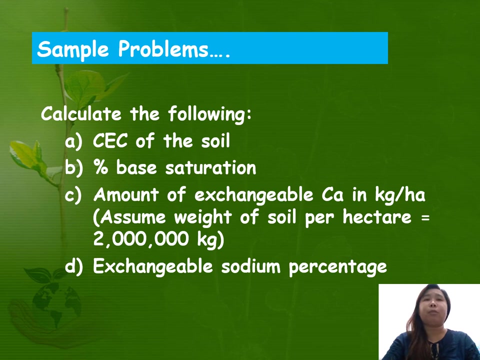 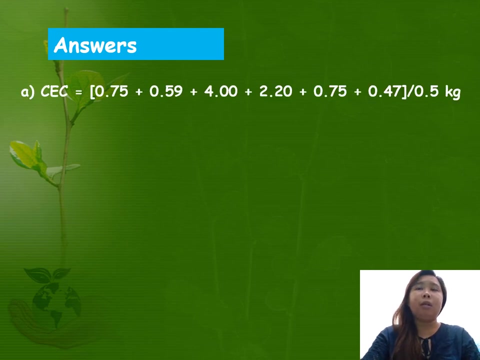 the following PEC of the soil: percent B saturation, amount of exchangeable calcium in kilograms per hectare- assuming that the weight of the soil per hectare is 2 million kilograms- and exchangeable sodium percentage. so let's answer this one by one. the CAC: we have the following data for the 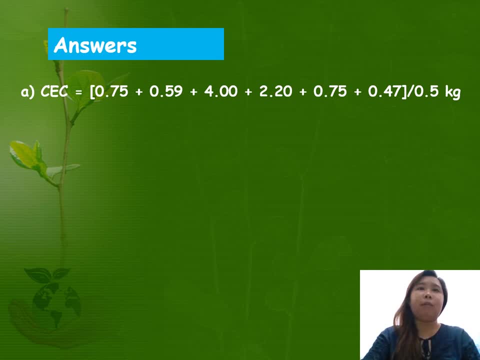 cations, that is 0.75, 0.59 for 2.2, 0.75, 0.47 centimoles. remember those cations that are mentioned from the previous video slide. so these are the values of um the CEC per um 500 gram or half kilogram of soil, that is 0.5. 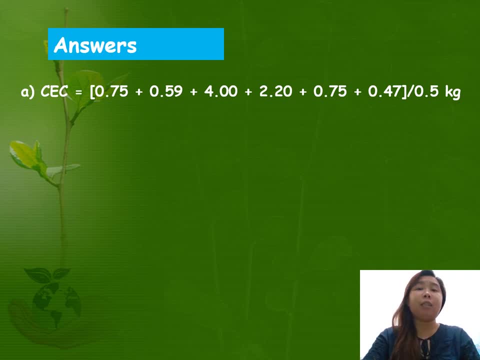 kilogram. now the unit for CEC is centimole per kilogram, meaning one kilogram. so how to answer this? just multiply all those centimole values by two, so you will have the unit of centimole per kilogram, because point 5 plus 0.5 kilogram is one kilogram. so 0.75 times 2 you have 1.5. 0.59 times 2, that is 1.18. 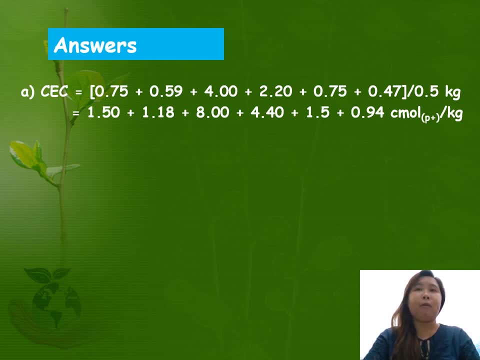 4 times 2, that is 8. 2 times 2, that is 4.4, 1.75 times 2, that is 1.5, and 0.47 is 0.94 centimoles divided by one kilogram. so the answer for CEC. 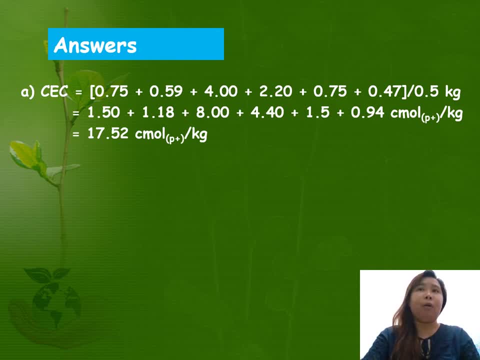 is 0.52 centimoles per kilogram. summing these values all up for the base saturation, that is percent vs. you just have to sum the bases and divide the value of the answer into the CEC value. multiply it to 100, that is 1.5- 1.8. 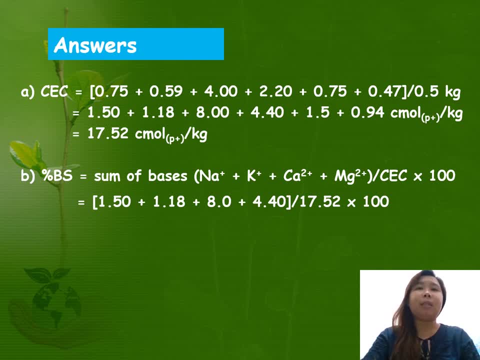 plus, rather 1.18 plus 8 plus 4.4. that is the centimole per kilogram or CEC values of sodium, potassium, calcium, magnesium ions divided by the total value of the CEC 17.52 multiplied by 100. the answer would be 15.08 divided by 17.52 times 100. 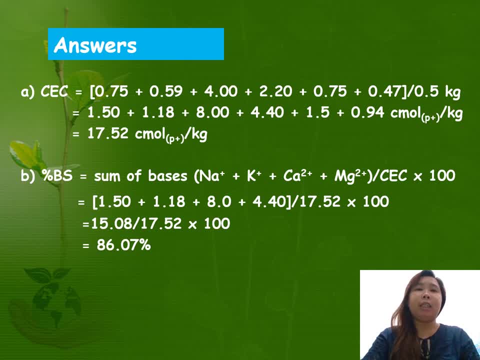 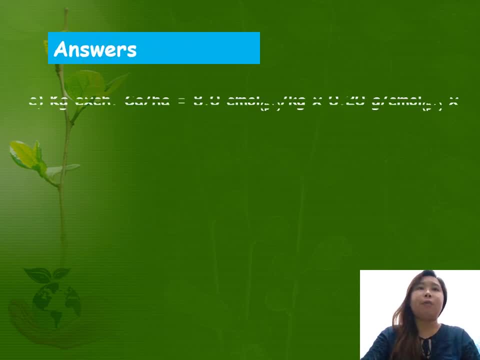 for base saturation. we have 86.07 percent that base saturation. now for the next problem. we have to calculate the um exchangeable calcium per hectare, the amount of exchangeable cation per hectare, that is in kilograms per hectare. so the CEC of calcium is 8. 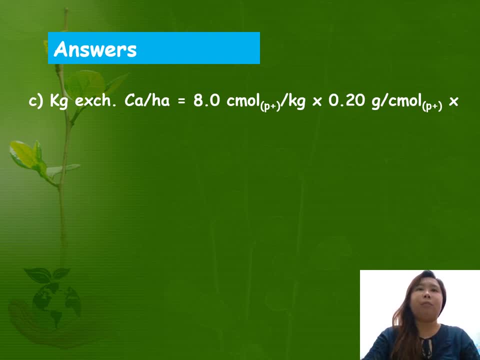 So we just multiply it by 0.20 grams per mole. remember, we have to calculate the amount of calcium per hectare. so multiply it by 2 million kilograms of soil- that is the weight of the soil per hectare- and then divide it again by 1000 grams. 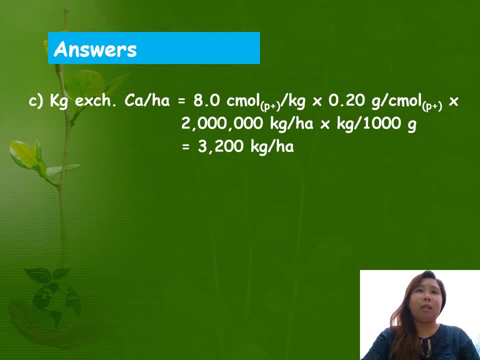 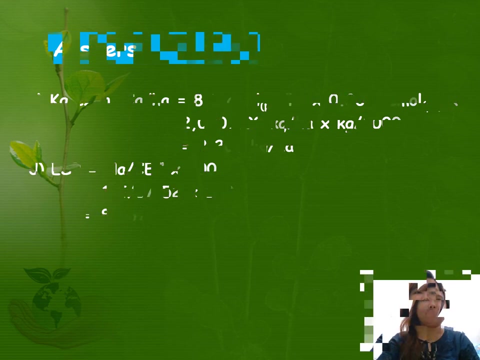 The answer would be: 3200 kilograms of exchangeable calcium per hectare are present in the soil. Now for the ESP, or exchangeable sodium percentage. we just have to perform this calculation or this formula. So the answer for the ESP, or exchangeable sodium percentage, would be 8.56%. 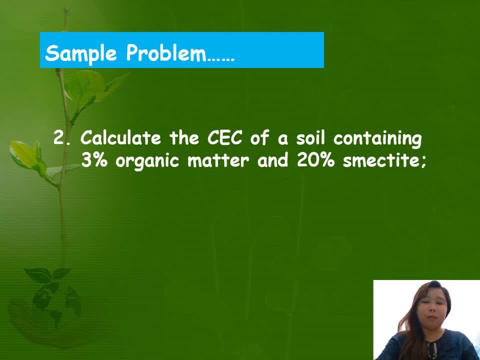 Now another simple problem: Calculate the CEC of a soil Containing 3% organic matter and 20% smectite. This is just similar to the previous problem we have, wherein the given data is about organic matter content and clay content.